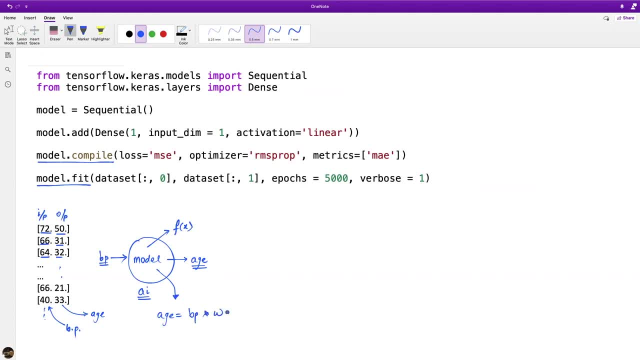 blood pressure times A constant weight plus a bias. So here's one metric parameter, another network parameter or the model parameter. But then basically this model is nothing but this mathematical function, where it simply takes the blood pressure as inputESM. unde司it. 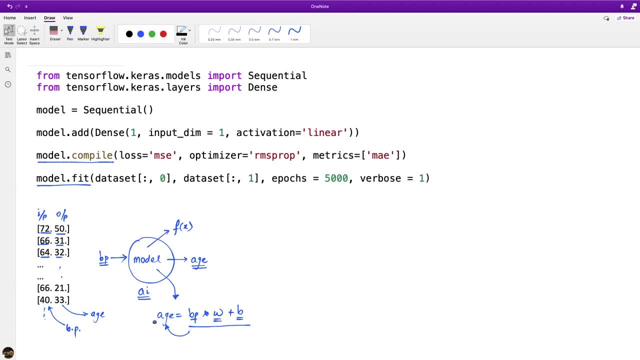 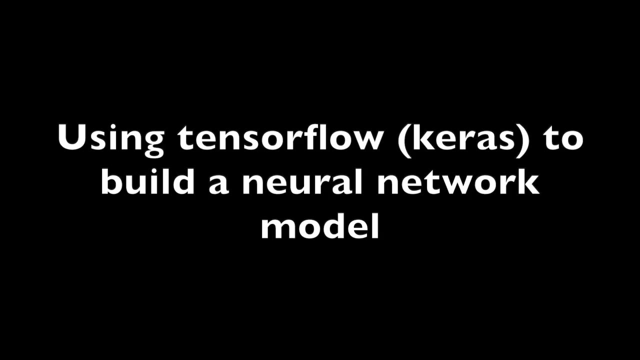 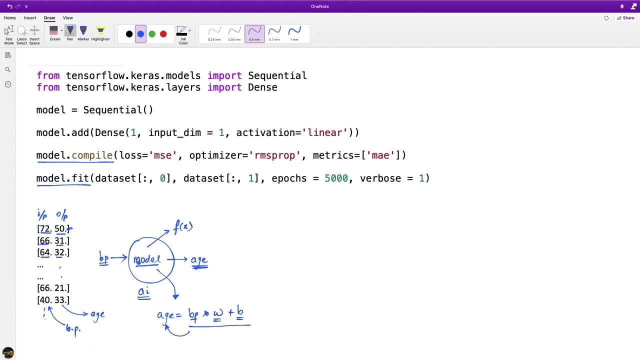 output a. So this is how the model makes predictions basically, And then the way we can make the evaluation of the model is by comparing how good the predicted is is against the true is when we actually have the true is at our hand. so to build such a model, where we create this model and automatically learn the weights and 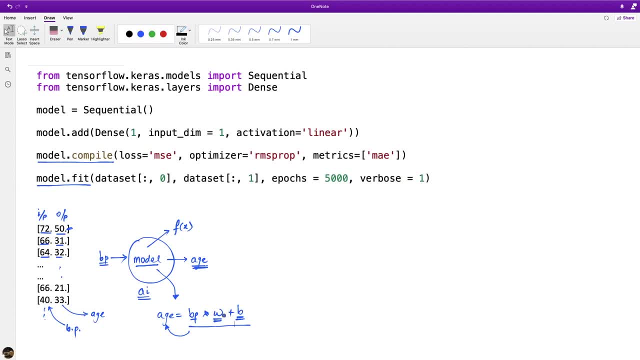 the bias parameters. this is how tensorflow can help us. the first thing we do is we import the libraries. in particular, for this case, we need two libraries. one is the sequential class in the models library from keras and the dense layer from the- the layers. now what the sequential class does. 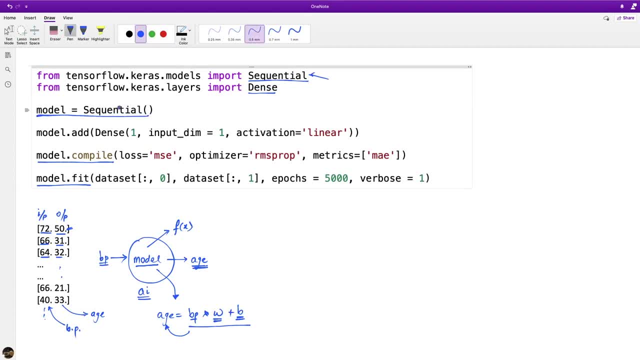 is allows us to build an empty model that's of type sequential. now why, um, sequential and and other other kinds as well? the answer is yes. there are other kinds as well. sequential is the type of model, where is it being constructed and by which you can create other models to build. 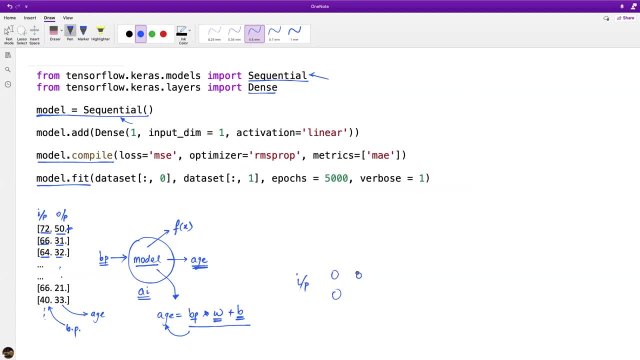 the model like this one. there is a sequence here which allows us to do this. if we want to express what sequence here? because this is the type of model that we want, the type of model that we want to apply, If you have your input, then the neurons. 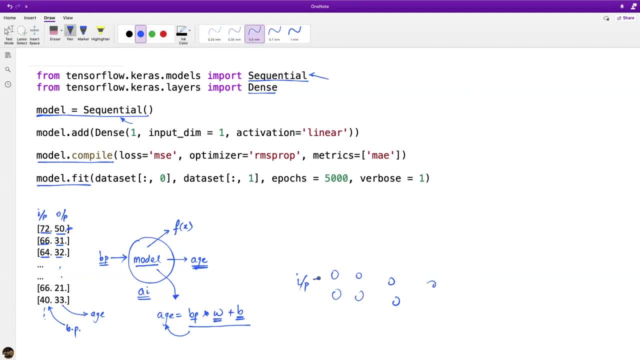 or mathematical operations that take place inside the model are always in like a sequential process. Your input goes in and they sequentially go all the way to the output for the output to be produced. So the other kinds of models could be recurrent architectures, where your neurons 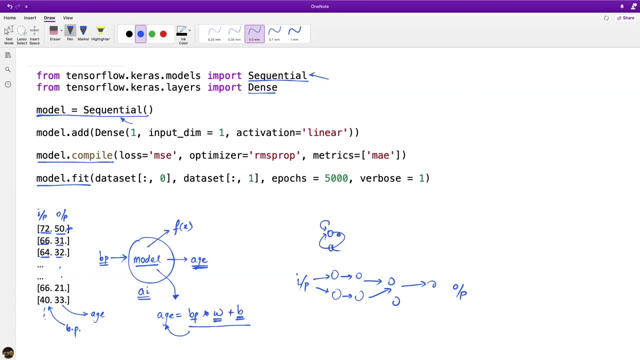 could be connected such that there are connections within themselves. there are cross connections and other kinds of connections where the input does not necessarily go from, say in this case, all the way from left to the right. There could be cross connections and other kinds of connections. 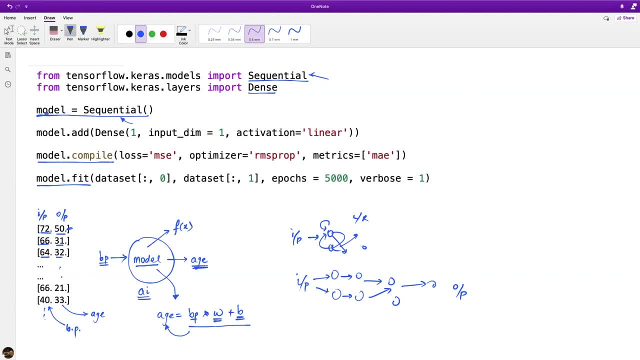 So those are non-sequential models. So the first thing we do is create an empty model that's of type sequential. The next thing we do is add a dense layer. So once we create a platform, an empty place for a model, for us to keep adding. 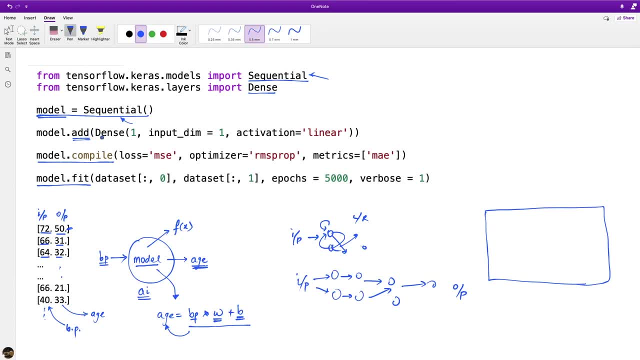 The first thing we do is add a layer called dense. Now, this word dense stands for a special type of network, And this network is something known as the feed forward neural network. Feed forward neural network: What this basically means is neurons connected in a feed forward fashion. 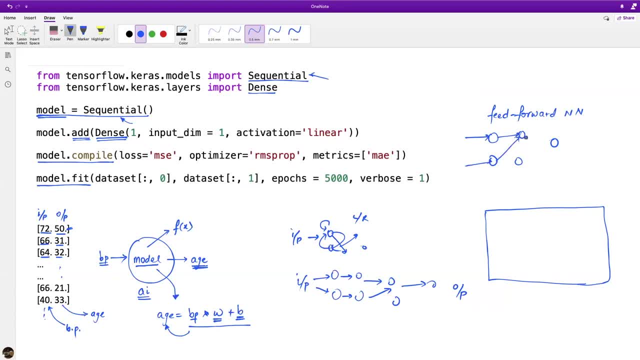 This is your input. the output from previous layer goes to the next layer and from the next layer to the next layer and then to the output. Now, in the dense layer, the parameters that we're specifying is one, So this one basically means that we have only one neuron. 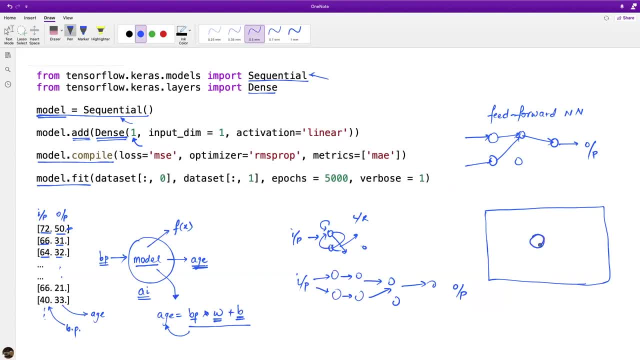 as our input. So one neuron means we have this neuron and it receives inputs. Here the parameter input dim equals one specifies that the number of inputs this neuron is going to receive. So I'm going to put that here. I'm going to put that here. 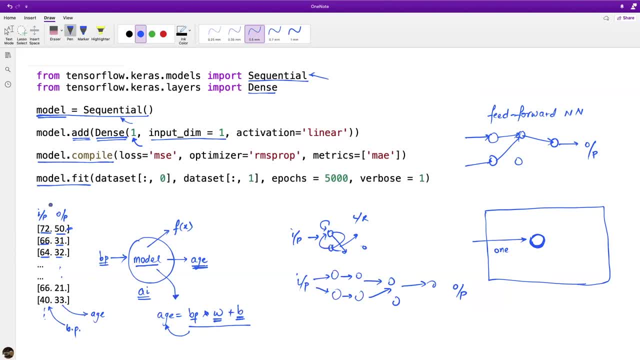 Okay, So we're going to use this one. So we're going to use this. one is only one, and this is the case because our input is only a single variable, one column input. so this, this model, only receives this densely, it only receives single input. in this place, the input is BP. we know that by definition of a. 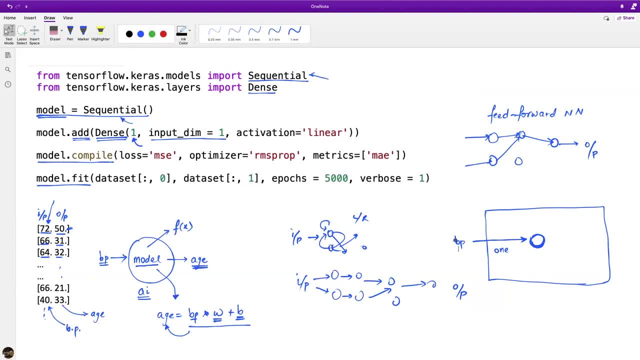 neuron on the way linear regression works. the input BP is going to be multiplied by a weight and a bias will be added to this weight, and then what comes out is predicted as the output. now this parameter activation equals the linear implies that no further activations are applied to this output. 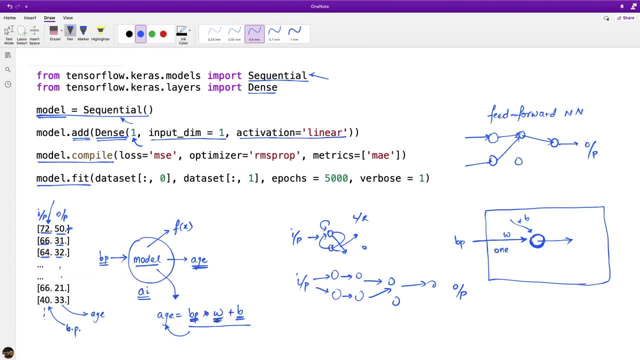 so this output that we have BP times weight plus bias, typically in a big neural network. what happens is this output goes as input to another function. typically it's either a sigmoid function or some other kind of activation. in other words, what this sigmoid function would do is take this as input and produce a number between 0. 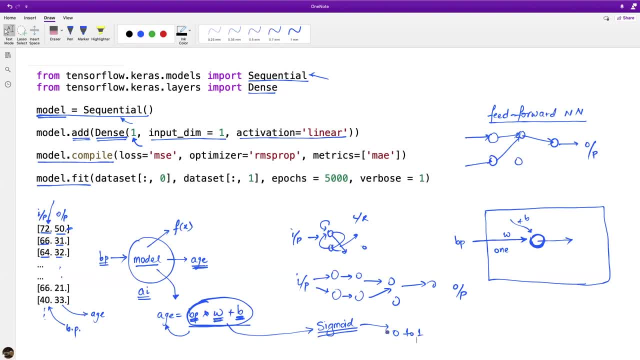 to 1. so these activations are, like you know, functions that take your models, some output, some input, and produce an output are absent here. so linear simply means we don't do anything. we simply multiply the blood pressure with the weight that the model has and we simply multiply the blood pressure with the weight that the model 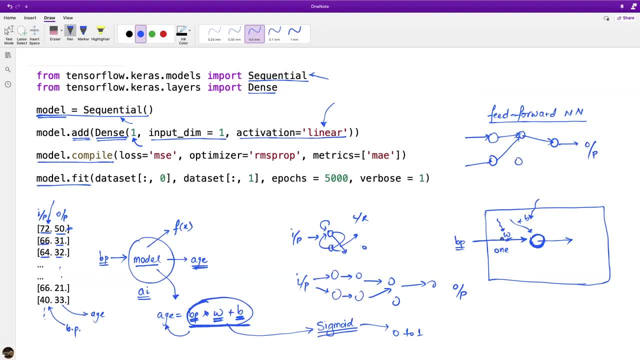 has to learn and the bias that also the model has to learn, and then simply produce the output without making it go through any sort of activation function. so up to this point, what we have done is we have built the model, we have built a model, and then the next thing we do is we do model compile. this process is to specify. 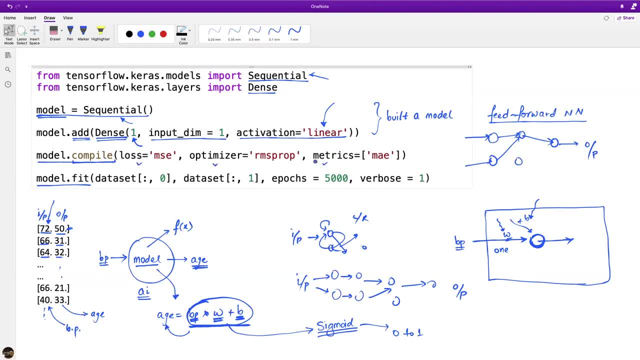 the loss optimizer, give some metrics, if we want, and also to check for errors if we have accidentally made connections that are not allowed in a sequential model. so this basically checks for the syntax errors in our process or even logical errors that we had in the process of building a model. now the first parameter: 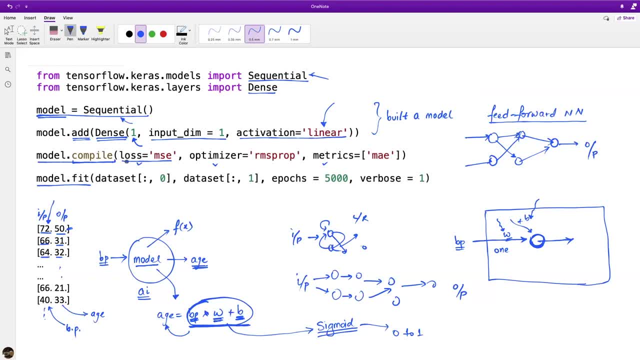 for calling the model that compiled function is the loss. so what this loss equals- MSC here stands is stands for- is MSC is mean squared error. so here mean squared error simply means as we build the model, we are going to pass the model the true output values as well, so that the model knows how bad the weights are. 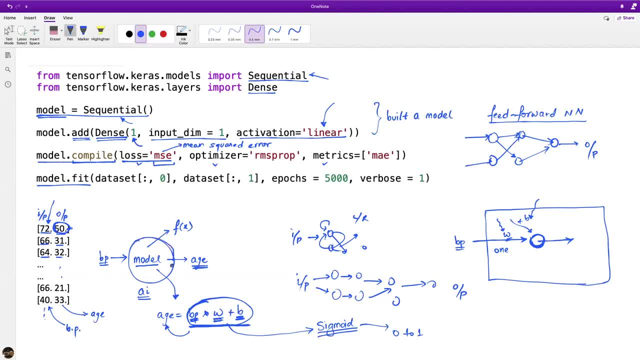 so and then it can update it right. so say, for example, we have this model and then we plus pass butt-presser error as input and let the model randomly initialize weights and bias to certain values and then also make predictions from the model. let's say we predict is P. 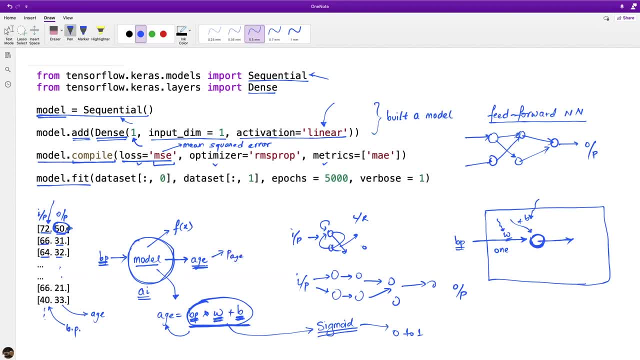 is so, then we also need to supply these values, which are P true, P true for the model to calculate the loss, to calculate the error, so that the model knows how bad its predictions are. and there are different ways we could calculate this loss. so this difference, difference. 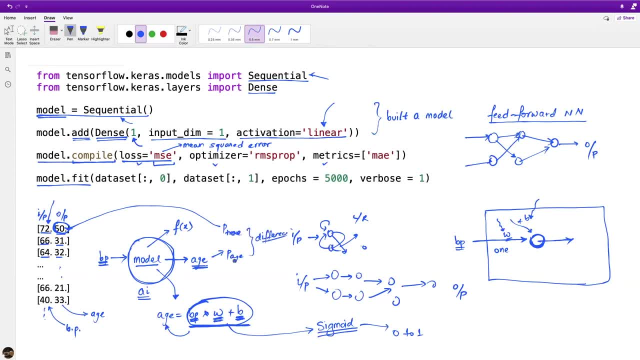 between the prediction and the true is is the loss, the error, and one way to calculate this is to simply calculate the difference, that is, absolute difference, between prediction and true values. another way to calculate this is to calculate the square of this error, and this is exactly what mean is square. 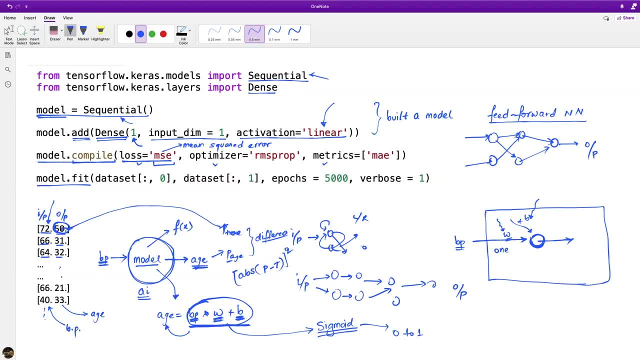 error means. so if this error is calculated between multiple, listing multiple examples, then this simply becomes mean. is quite error. now, with loss equals to mean, is Got Error. what we are telling the model to do, two figures is one data- 2, 4, very useful to I. 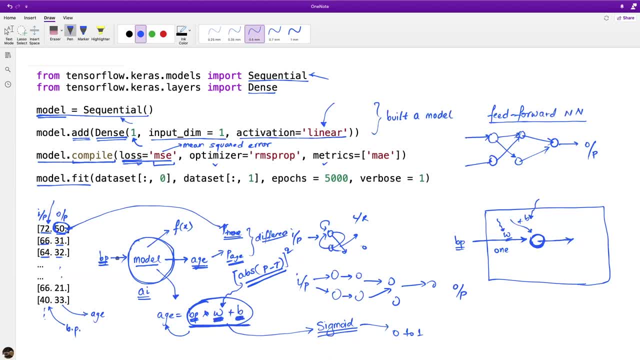 say 9, 10, its weights and biases so that in the future the model makes better predictions. and this is an iterative process. Now, this parameter optimizer equals RMS. prop is the algorithm that your model uses to iteratively update the weights. So the way weight updates work, or it's specifically in the case of neural, 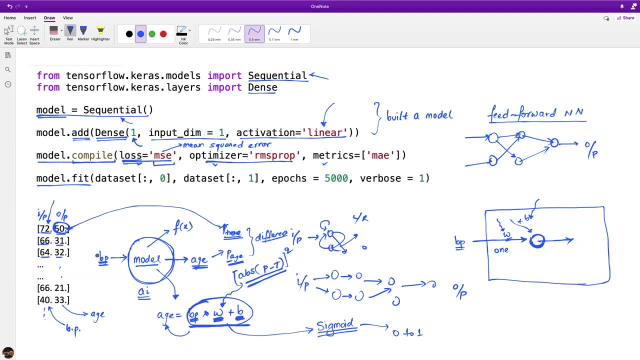 networks. back propagation algorithm works. is your model. takes certain blood pressure as input input, makes predictions, calculates the loss, updates the weight and bias values and then makes predictions for remaining data or for subsequent data. again predicts the output, again calculates the loss, again updates the waste and then goes back, makes further predictions and continues. 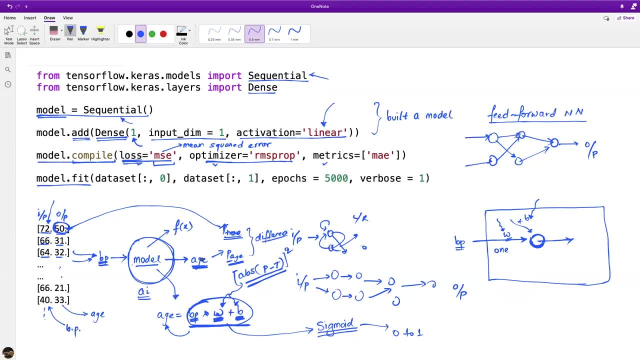 the cycle. So this cycle of taking the input, making predictions, calculating the loss, updating the weights and making predictions using the weights that are updated is a iterative cycle and it does the and the model. we would like the model to do this continuously until no further weights and biases can. 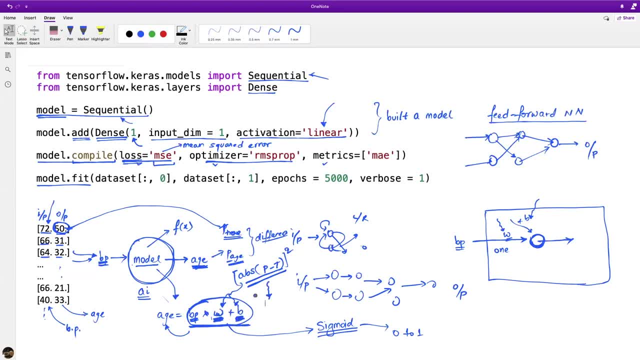 be updated to get lesser and lesser loss right. So this back propagation algorithm, the process of updating weights, is controlled by your optimizer. There are various kinds of optimizers. RMS prop is one of them. there's Adam. there's an Adam, there's a S. 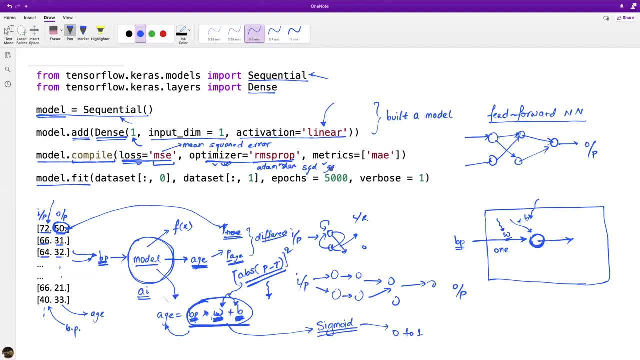 S, G, D, There's gradient, decent and so on. so RMS prop- usually there are around a dozen or so these of these kinds of optimizers and RMS prop user. it pretty much works for the most problems, at least at the beginning when we are learning machine. 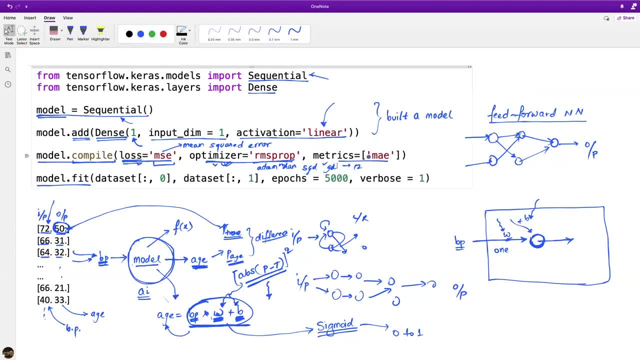 learning. Now this parameter metrics. it's simply informing the model that compiled that as you perform these weight updates and then every time you do these weight updates, you might want to report us How bad the prediction size. so, Amy, is simply the absolute difference between the predictions and the true. So this is mean. 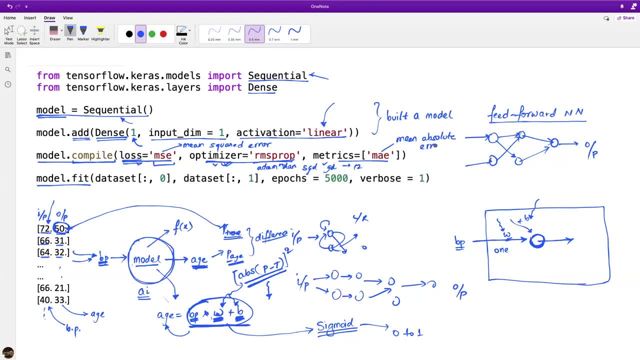 Absolute They're. So any simply calculating the difference between the true out, the true that we have and the prediction that we have now with metrics, equals my. what this model is going to learn or no is in future as it to reports its performance during the process of learning. it's going to simply calculate mae and report that. 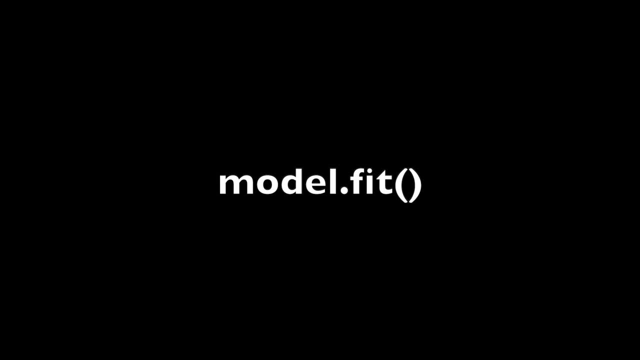 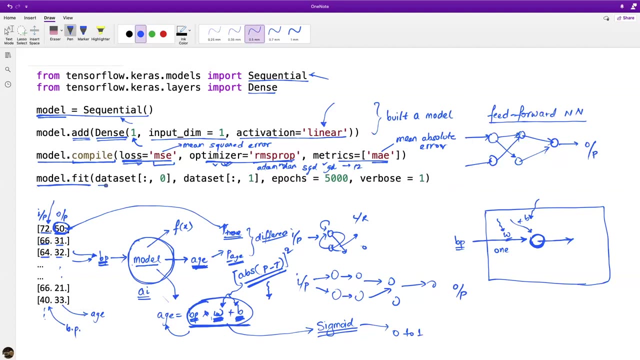 to us now the last function, modelfit, has a lot of parameters as input: 2.. the first parameter that we supply as input is the x, that is the input to the model. so this is where we specify. take this column that we have as input. so this is all rows, the first column and the second parameter. 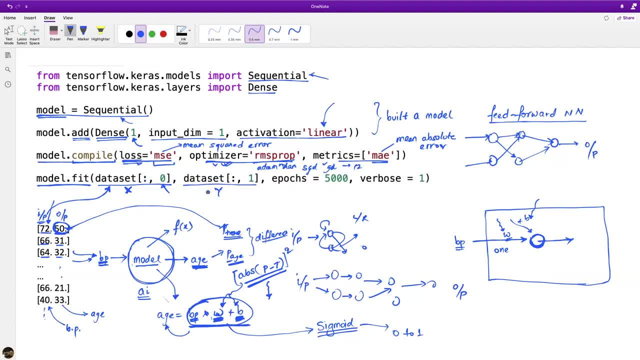 is the y for our model, that is, the actual labels that we want to provide the model. so these actual levels will provide the model so that the model can calculate the error during the time of learning. later, when we actually use the model to make predictions, we don't supply y because at the time of making predictions we don't know the. 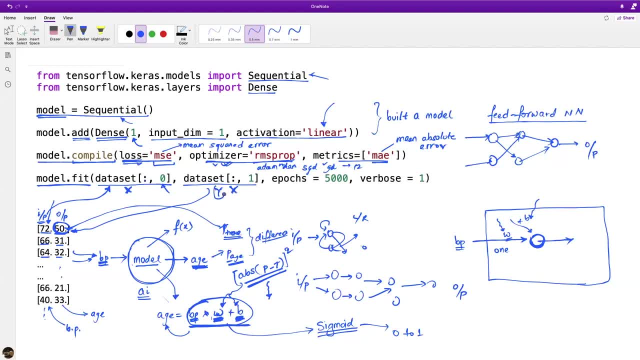 truth of the model. when we actually use the model, we don't know the truth of the model, true value. so this Y is supplied to the model only during the training, that is, when we call the model that fit process. now the next parameter we have is epochs. 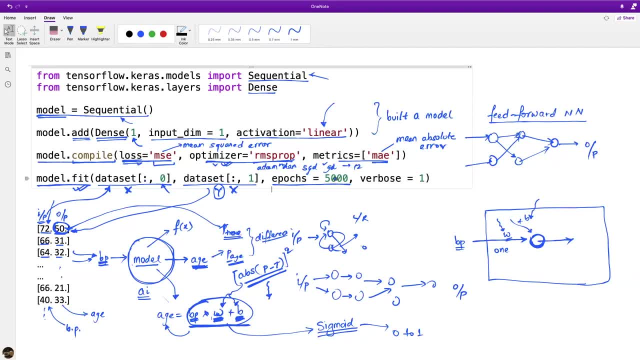 so this epochs is the number of times, number of times, times. we want the model. we want the model to see the entire data set. the entire data set, in other words, if we have epoch equals 5000. that means, during the process of doing these weight updates, that is, updating the weights and building the model, our model sees the 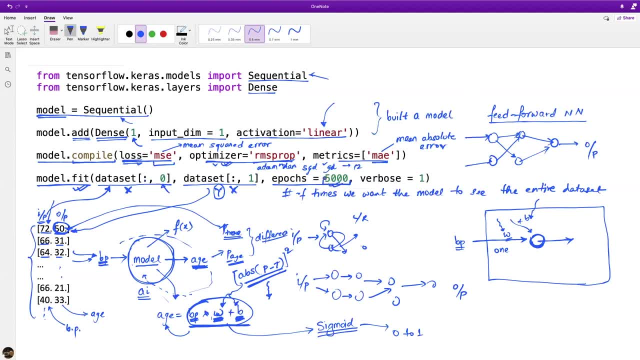 entire set of data five thousand times now, even in one epoch, even within a single epoch, in one epoch the model might split the data. so if I have 1000 rows of data, the model may look at 32 examples at a time. so look at 32 examples, update the weights and then go. 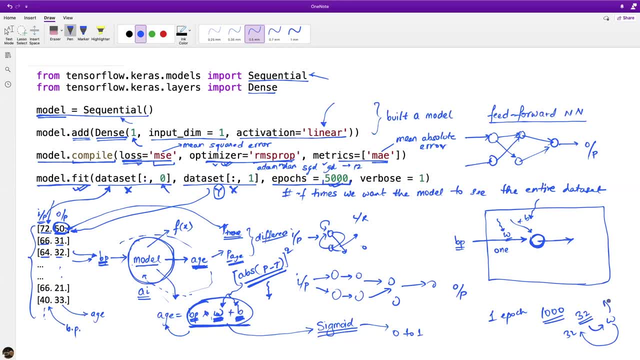 back, pick up the next 32 examples, update the weights and go back and fix- not pick next 32 examples- and so on until it has looked, scanned through the entire data set. so this all happens in a single epoch. so in one epoch the model looks through the entire examples at one time and this parameter is known as batch. 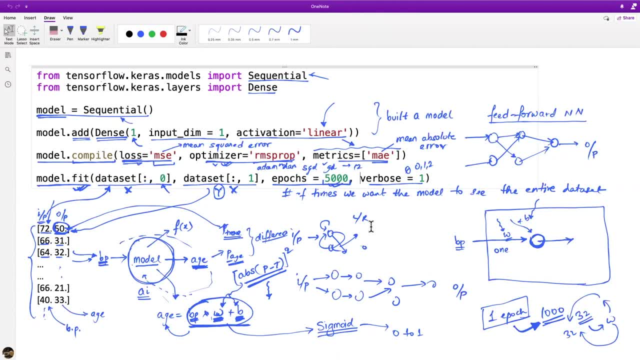 size and we can specify that size when calling modelfit by simply putting batch. underscores s eye's equals whatever number we want as an additional parameter in the model dot fit function. so, but I think by default it's 32, but we can specify smaller of batches when calling the modelfit function. Now, larger batch sizes may make. 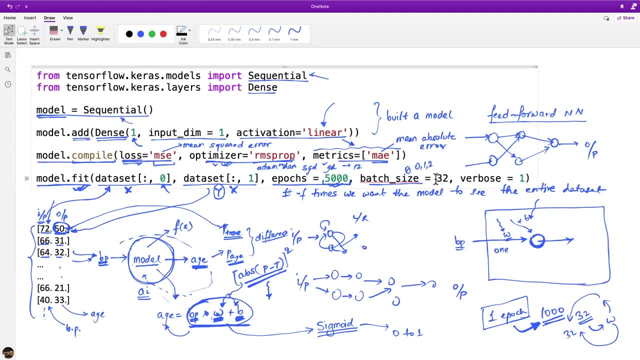 your training run faster, and smaller batch sizes may make your training go slower, but then usually leaving it to numbers like 16, 32 works very well. The last parameter- verbose equals one- is simply telling the model whether or not we want the intermediate outputs to be shown in the screen as we 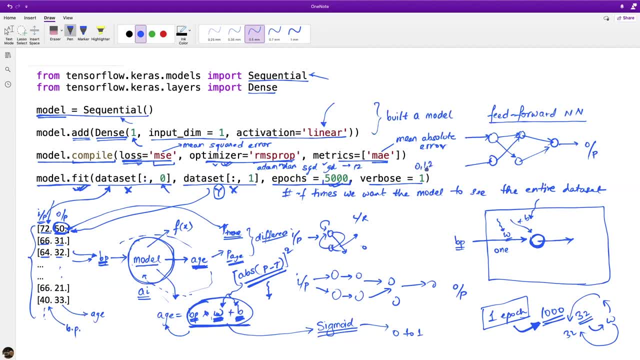 run the modelfit. The options are 0,, 1 and 2, depending upon how verbose we want. For example, if we specify verbose equals 0, then this heap right here does not have a lot of meaning because we don't. we will not be able to see the MAE, while the training is happening.